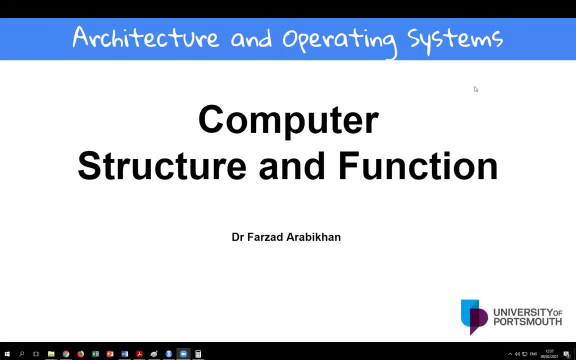 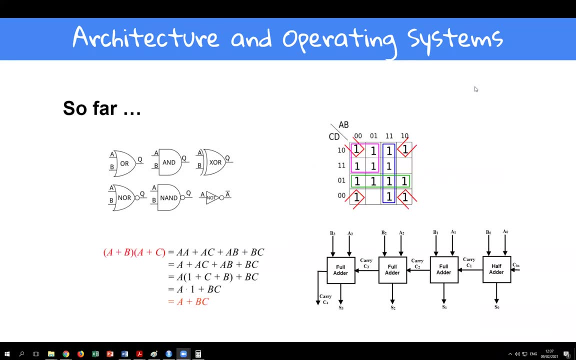 Hi everyone. Architectural Operating Systems and we are going to start the second semester of this module. In this semester we are focusing on computer CPU function structure and also operating systems. What we learn in the first teaching block will help us to understand the stuff and topics in the second semester. 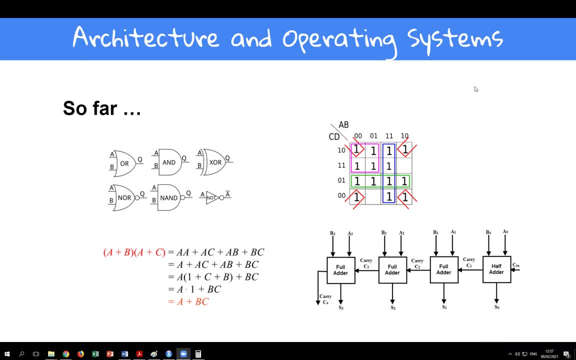 In the first teaching block we learned about binary numbers, how to translate different different numbering system into the binary and how to use them to do the operations, arithmetic operations like addition, subtraction and so on, And also we learned about logical gates, how to create a circuit to be able to do those operations like add or subtract. 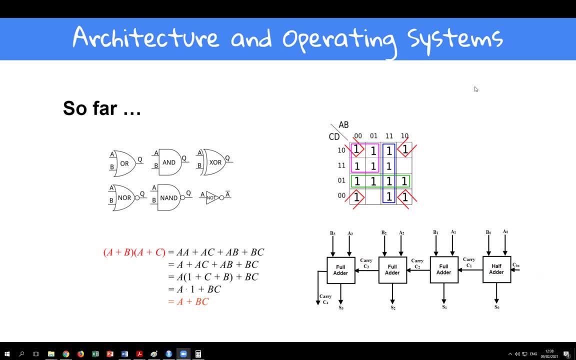 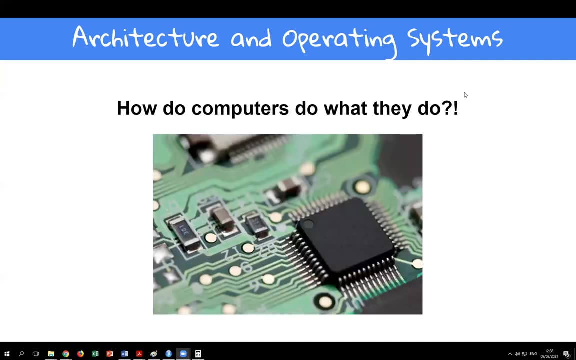 Not only that, we learned other techniques like coronal map and Boolean analysis. We also learned algebra to optimize them. Now in this semester we want to see how to use this stuff inside the CPU to do the operation. So this is the question: How do computers do what they do? 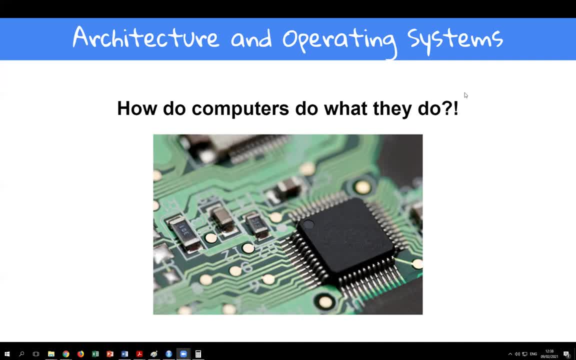 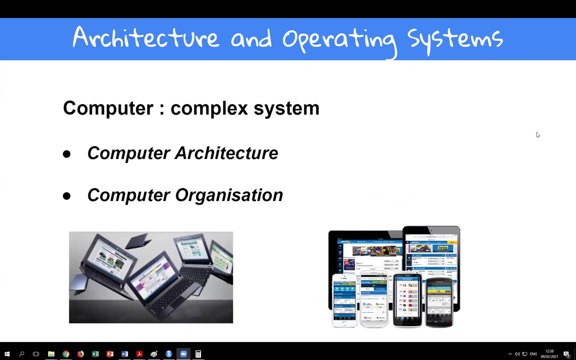 We want to understand when you want to add two numbers. you know what happens inside the circuit, But what happens inside the computer using different components to do this addition? This is our focus. So computer is a complex system. Complexity means that we've got different components and we've got to put them together in a logical way to be able to undertake different operations. 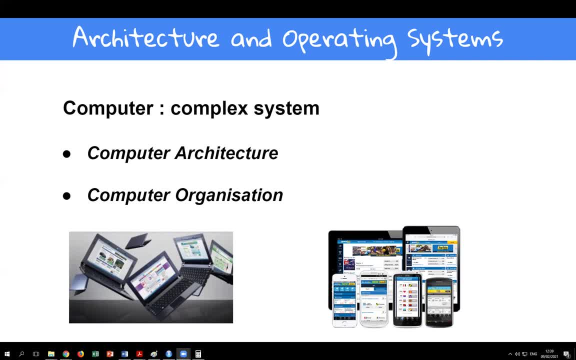 But first of all we need to learn about computer architecture and computer organization. So first of all, what is computer architecture? Computer architecture refers to those attributes of a system visible to a programmer, Or, to put it in another word, these are attributes that have a direct impact on the logical execution of a program. 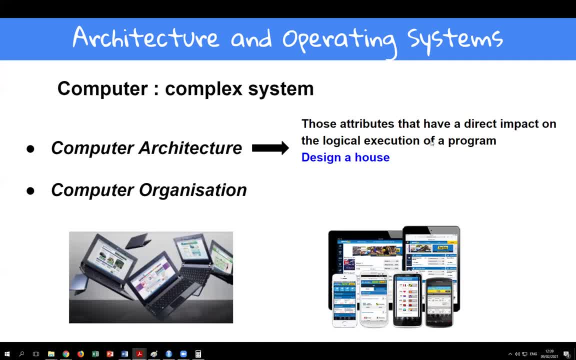 So, as you see here, computer architecture is like a design house. When you want to design a house, first of all you need to draw a floor plan. And where is the kitchen, where is the toilet and where is the different parts of the house? 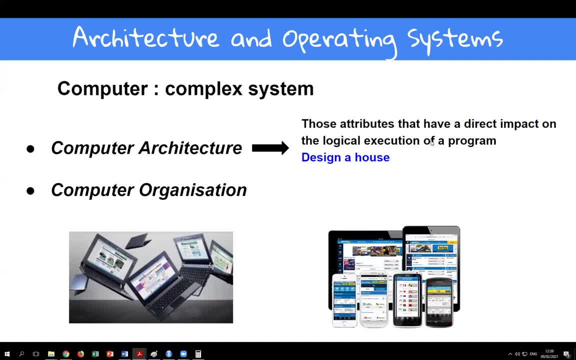 You don't think about the components at that level. So the computer architecture talks about this, That how we've got to use different components, but in the logical way to be able to execute a program. So it's like a design, a house. 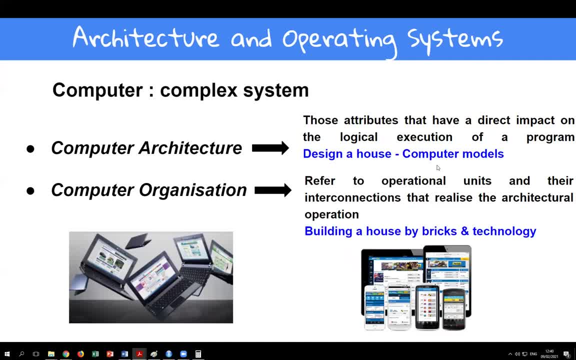 But computer organization refers to operational units And the interconnection there to realize the architectural operation. It means that it's like building a house by bricks and technology. So first of all, using architecture, you've got to design your house and then use bricks and different technologies and other stuff to build that house. 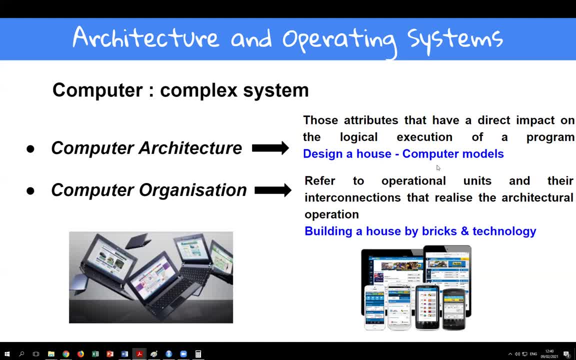 So this is the difference between architecture and organization. In architecture, Logical execution of program is considered. In organization, different components and units need to put together to actually do the operations. So look, guys, as you see, for example, in the mobile phones here, I think it's better to do it like that. 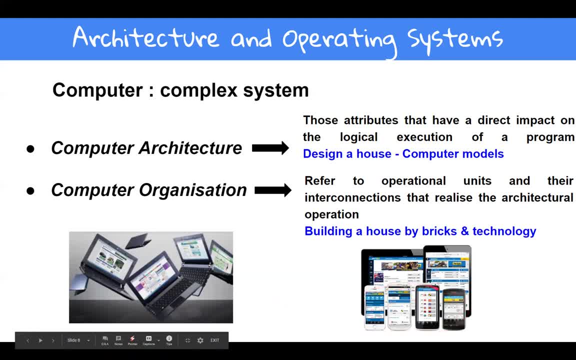 In mobile phones, all of them have got the same architecture, But we use different components, different organizations. In Apple mobiles or Android mobiles Tablets, they have different architectures And different models, use different brands, use different organizations, But they have same architecture. 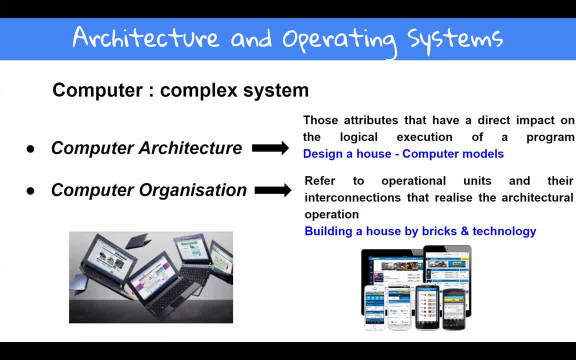 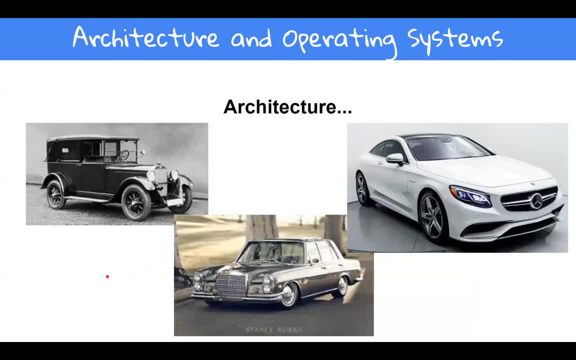 Same is true for the laptops: Most of them use the same architecture, But the components and units are different. Better example: Mercedes, Mercedes, As you see, from this machine, which is very old, to the newest one that we have here, and actually the middle ages of them like this, most of them, actually all of them, have got the same architecture. 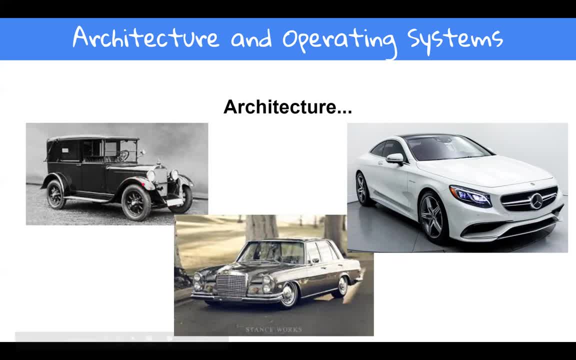 We need to have wheels, We need to have engine, We need to have gearbox, We need to have different parts that they've got, to put them logically, to be able to actually run this machine, run this car. But definitely the organization and components of this one is totally different with this. 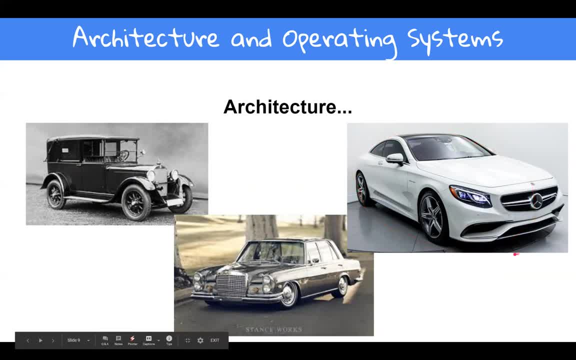 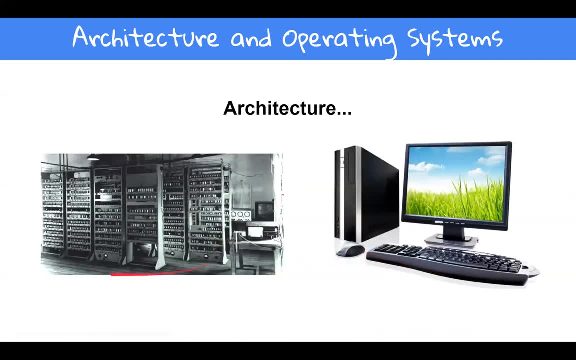 And totally different, is different with the newest one, But same architecture but different organization. So this is one of the first computers that we have And it's quite interesting to let you know and tell you that this machine that is quite new and we use it these days. 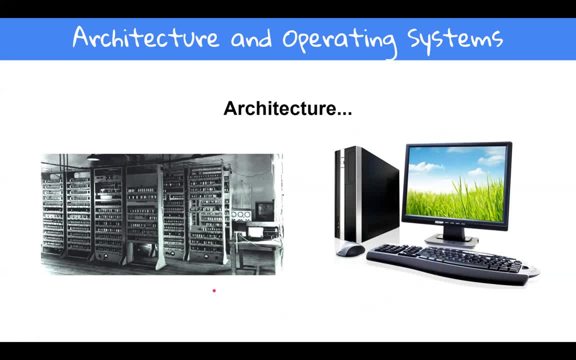 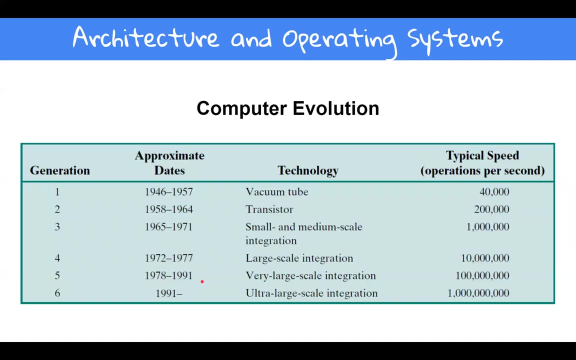 Has the same architecture of this very old machine. So today I'm going to tell you what is the architecture of the machine and how it should be. But the organization and technology has changed. For example, the first machine- 1946, that will tell you what machine is. 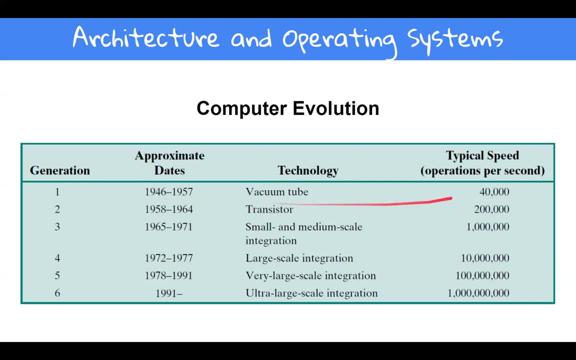 It used vacuum tube And the speed is like this: 4,000 operations per second. After that we are in multiple core CPUs that we can actually operate, And we've got super machine and even cloud machines that they can do loads of operations and in a very higher speed. 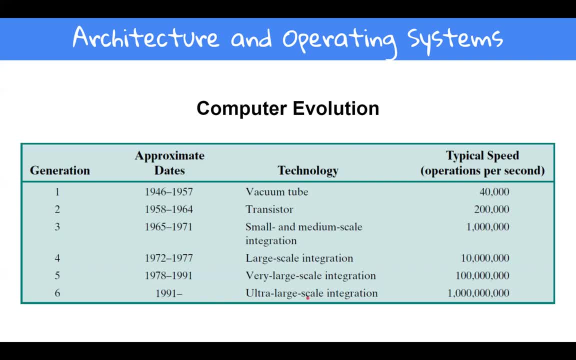 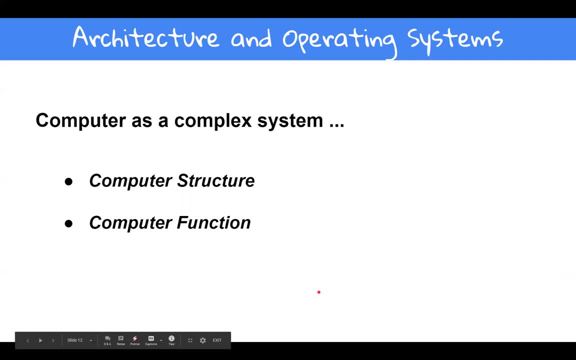 But all of them have the same architecture. This is about the organization and components. So computer has a complex system. Computer has got two different parts. Or, if you want to study, it's better to focus on two different things. One of them is computer structure and the other one is computer function. 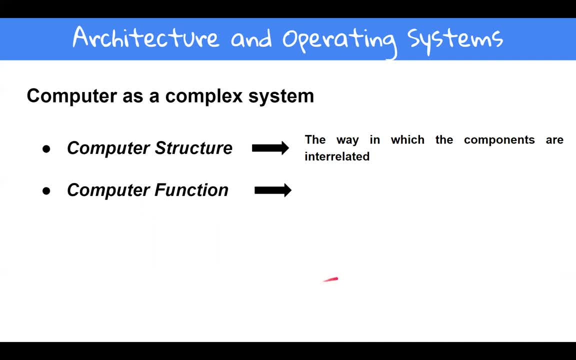 Computer structure is the way in which we, in which the components are interrelated. You're talking about how the components work together, Function, the operation of each individual component And each individual component as a part of the structure. It means that first of all, we need to study the structure and see what are the different components. 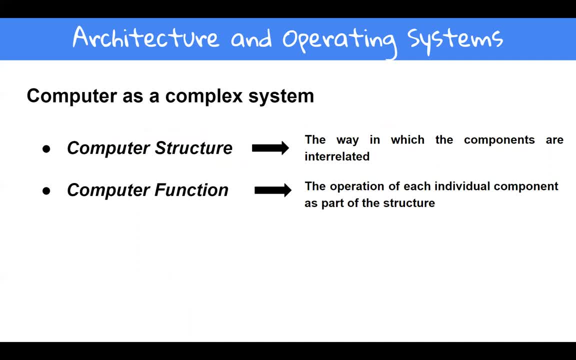 How to put them together, like memory, like input-output devices, like CPU, ALU. I'll tell you all of them. Different structure got to put them together, But the function is how and what each component does. But I want to start from function first. 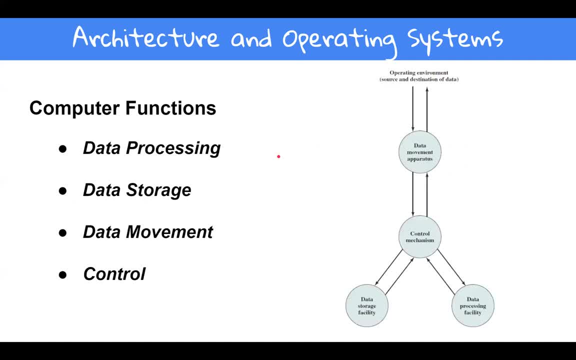 What are the main functions of our computer Computer, generally speaking, two full main operations and functions: Data processing. Data processing is in this part of the machine, That's our graph here, So it processes the data. So you know that in the adder or subtractor that we discussed in the first teaching block, 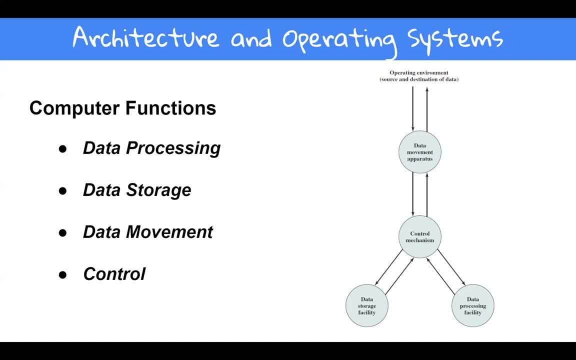 we know how we can use logic gates, put them together, create a circuit to do the operation So we can process the data here. Storage data: We must be able to store the data. If you want to add two numbers like four plus five, 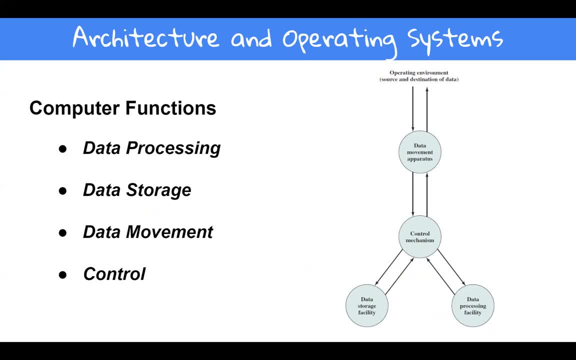 OK, you've got to store the first number and then store the second number, Do the operation and then store the output. So, data storage: We've got temporary data storage, We've got long-term data storage And we need both of them. 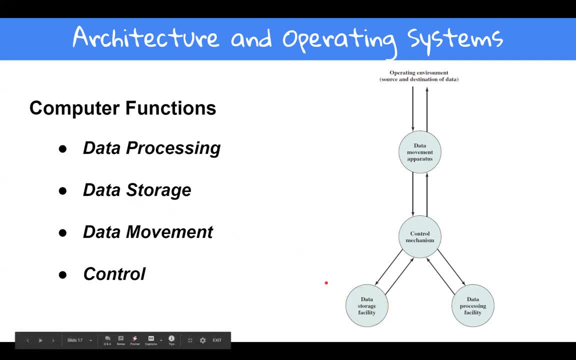 So data storage is another thing. When you save a file on your machine, actually you are using the storage capacity and facility of your machine. Data movement, Internet Data communication: You send the data, You receive the data, The data movement between different parts of the computer. 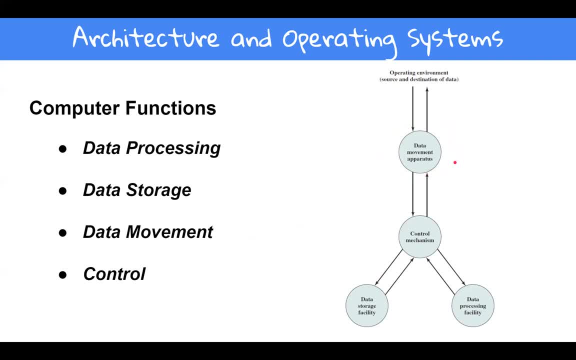 All of them is data movement. It's a function of our machines And, at the end, someone should control this machine. It's a control mechanism or control system, which is the most important part of that. When you write the code for your machine using Python, Java, different languages, actually, you are helping the machine to control the instructions, the program. 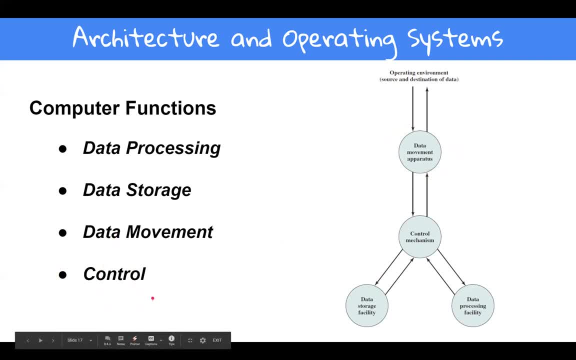 So control unit is very important. We will focus on that and discuss it in more details later. Data processing: When you want to process the data, definitely you need to be able to store that. Add two numbers, Get the first data. 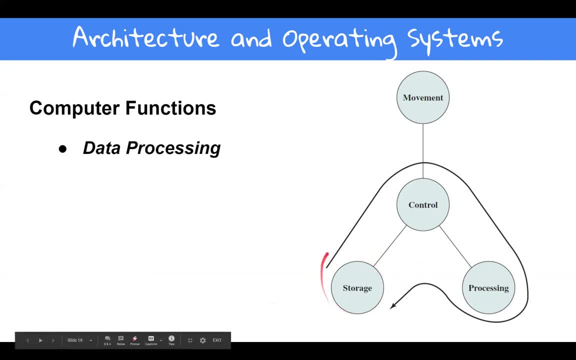 For example: two: Get the second data. Four: You've got to store them first And then, using the control unit there, actually send it to the processor to process it, Give it to the other subtractor. When you do that, when you do the operation, send it back to the storage. 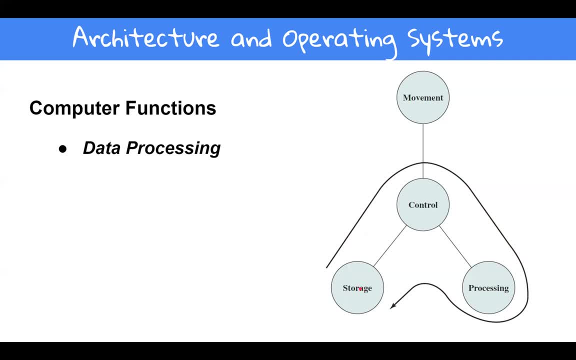 Because we don't want that. We've got to store that data, Otherwise we cannot display that on the monitor, for example, or cannot send it to the printer. So we need to have control unit in the middle. Data storage- Long-term and short-term. 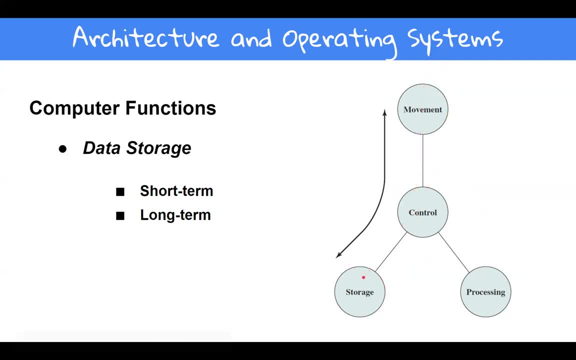 I told you, From the Internet you get the data. You've got to store it. You are getting a website. You are getting the data, The data movement, Data storage, Long-term and short-term. You want to add two numbers. 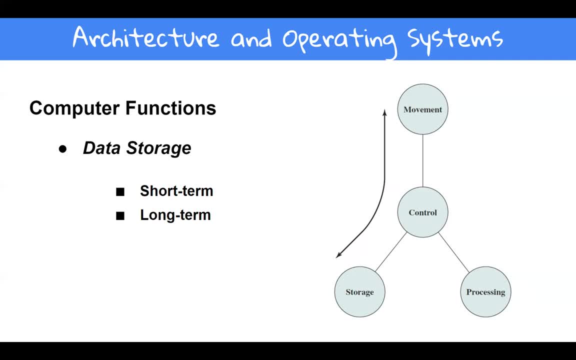 You need only short-term memory or data storage, But if you want to save it on your hard drive, it's a long-term. Again, we need data control unit in the middle Data movement. You want to send and receive the data. 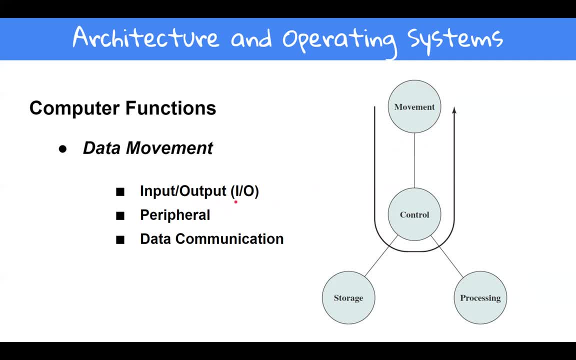 Data movement Input-output devices, For example scanner, Keyboard, Monitor, Loads of other input-output devices, Or we call them, generally speaking, peripheral components. They stop the other external devices that we have That we use And also we've got data communication. 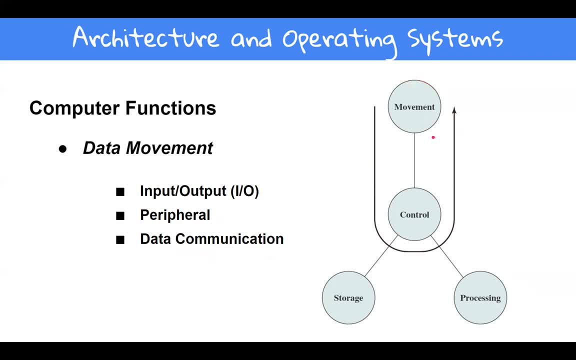 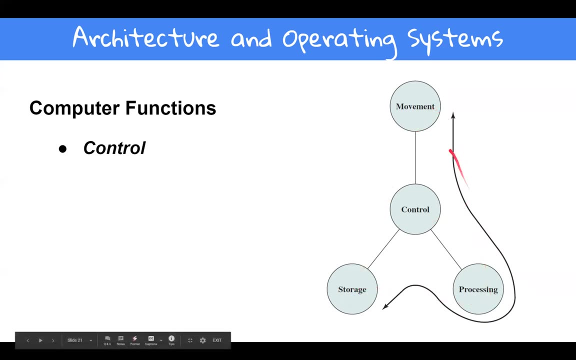 Internet. All of them happens here In the data movement function of the machine. And again we must have control unit in the middle to be able to control all of these operations. Control unit- The most important part- that actually handles the data movement, timing, everything. 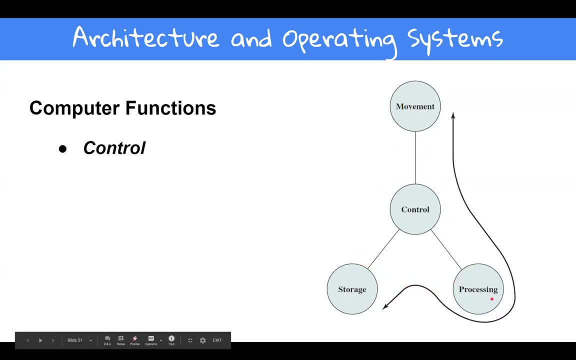 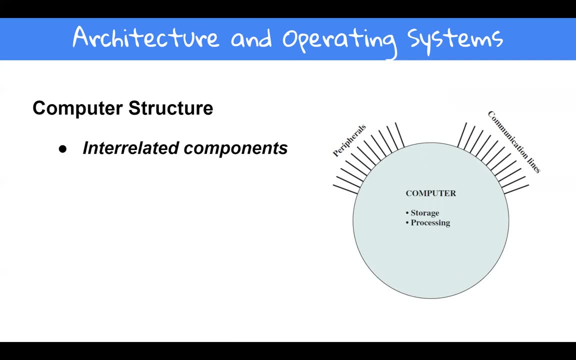 Everything between these four components of the machine. Now we know different functions of machine Components. Generally speaking, the computer structure. it's about the interrelated component. This is the computer. We store the data And we process the data here. 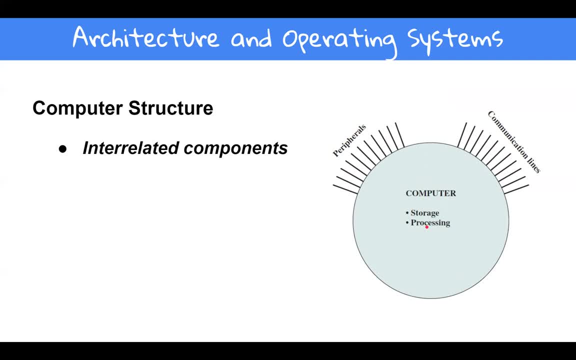 We process the data always at this time Actually remind the other subtractor, We use that as a processing unit, Storing the data here as well. But we've got loads of peripheral components Like keyboard, Like a scanner, Like printer. 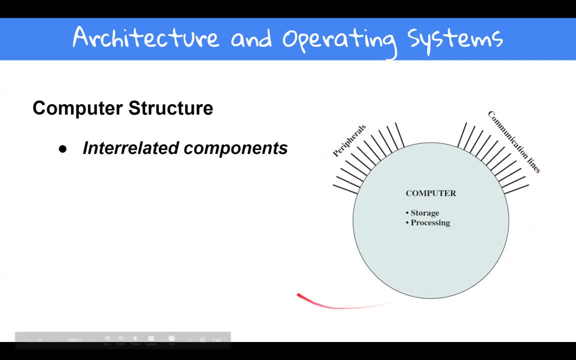 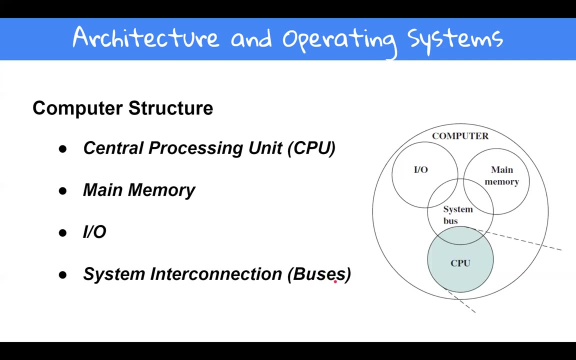 Communication lines. So, as you see, these are the four main components, interrelated components of the machine, And we call it computer structure. We will discuss that in more detail shortly. So, computer structure: What are the main components that we need to have inside the machine? 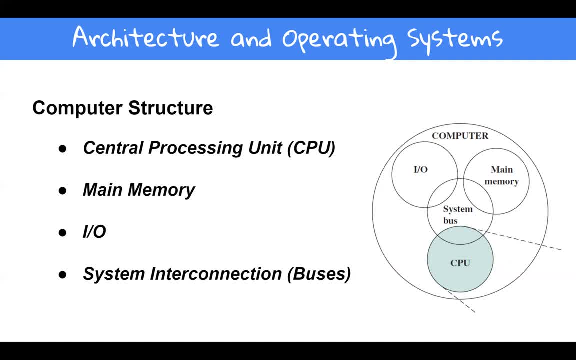 The most important one that we have is called central processing unit, Or CPU. CPU actually does whatever we want to do, And it controls the operation of the computer and performs its data processing function. We simply refer it to as processor, So whenever you hear about processor, it means that we are talking about the central processing unit. 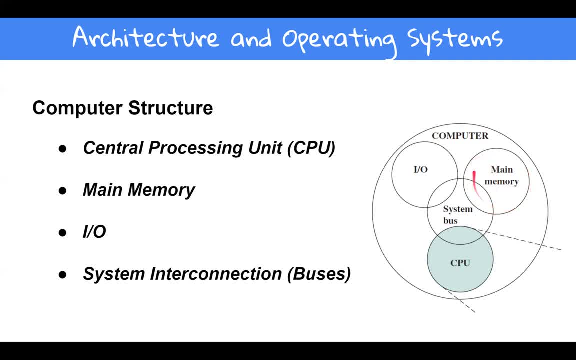 Then we've got main memory here. Main memory is the memory that we store the data If you want to get, for example, if you want to add two numbers, four and five- These four and five in the first place they need to sit inside the memory. 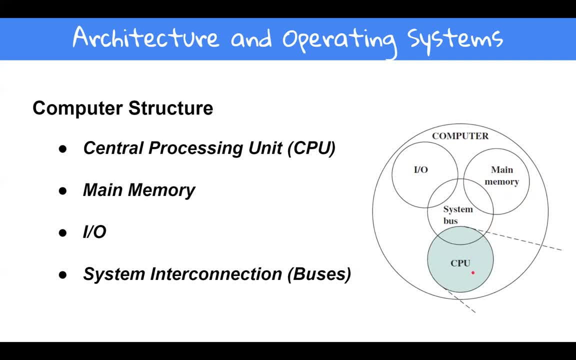 Because we need to have a place for them And then send it to the CPU to process. the data Input output devices is where you write the code. How you write the code Using the keyboard. Where do you see that On the screen? 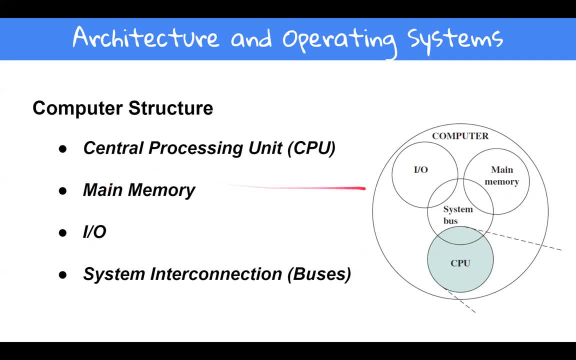 When you execute the code, where do you see that? On the screen, Input output devices? Or on the computer, On the top level of computer structure? And also we need to have a system to communicate the data between these three components. 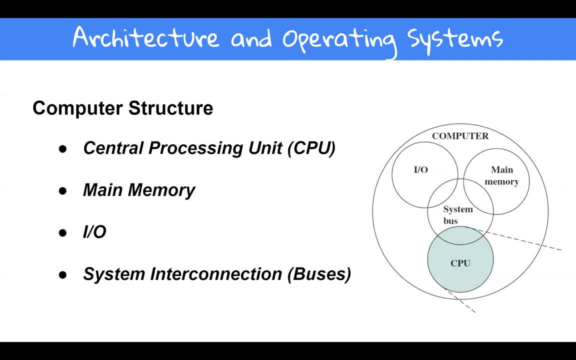 Some mechanism that provides for communication among CPU, main memory and input output devices. A common example of system interconnection is by means of a system bus, As you see here, Consisting of a number of conducting wires To which all other components are attached. 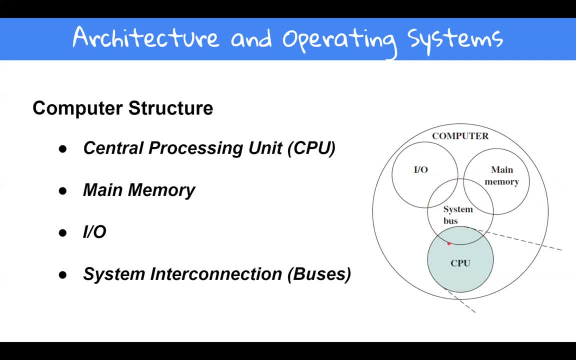 So all of these components are attached to this bus And we will discuss that in one or two weeks time. That how send and receive the data between different components. So this is the top level of computer structure. Now we want to focus more on the CPU. 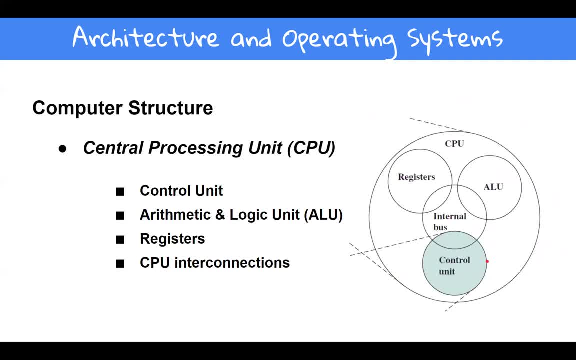 And see what we have in CPU. Let's look at inside the CPU. So inside the CPU We've got different components. What are they? One of them is control unit. The most important part Controls the operation of the CPU and hence the computer. 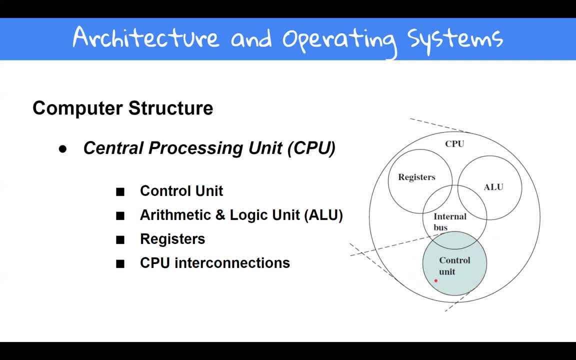 So this is the brain of our machine. How it does that When you write a code, When you write input X, It sends a signal that everyone should be ready. We are getting a number. So this control unit send signal. 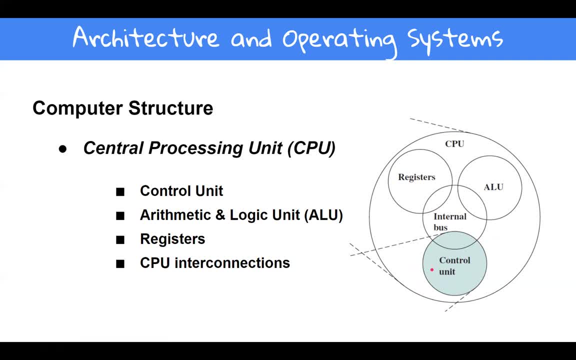 By sending the signal Controls different components of the machine. We've got arithmetic and logic unit, ALU. Arithmetic and logic unit Performs the computer's data processing function. You know that very well. This is the part that we focus in the first teaching block. 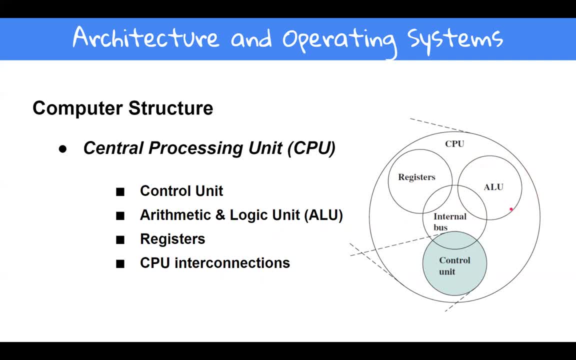 Because we know that, how computer Put different logical gates together To do operation. Not only that, We need to have the most efficient circuit. Again, we know how to do that. So this part is what we focused mainly in first teaching block. 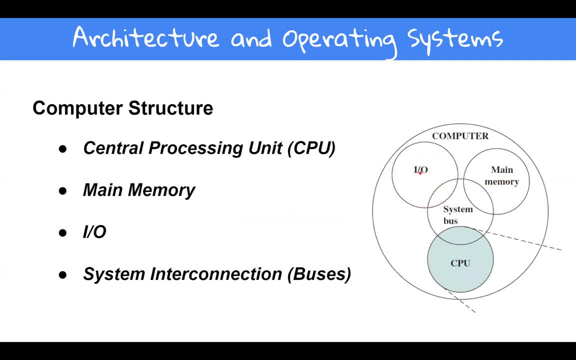 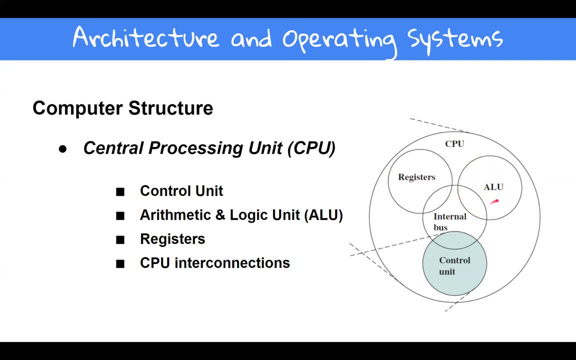 When using this input algorithm device That you put two numbers like two. First of all, This ALU converts that to the binary And put it inside the other circuit that it has And do the operation for us. Then we've got registers. 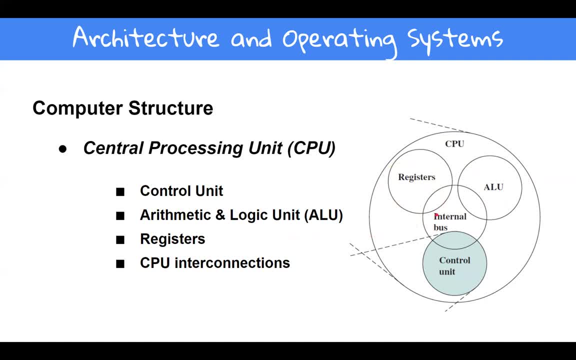 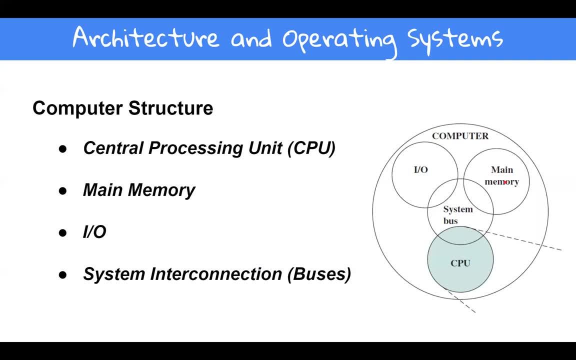 Registers Or internal memory of our CPU. When you get a data here, It goes first of all sit inside the main memory. Maybe we've got loads of numbers there, But those numbers that we want to use Using this system, We bring it to the CPU. 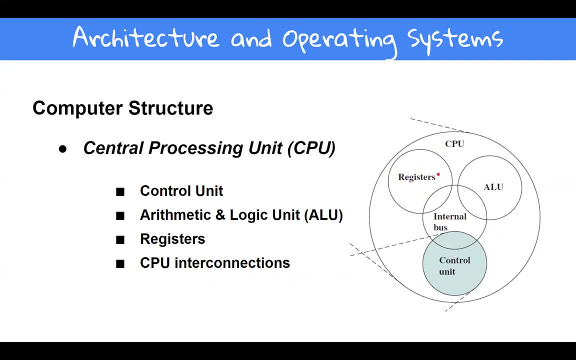 So we need to have a space to store them. This is called registers. Different type of registers Will be discussed later. And then, Between these four components, We need to have some sort of communication too. This is called internal bus. 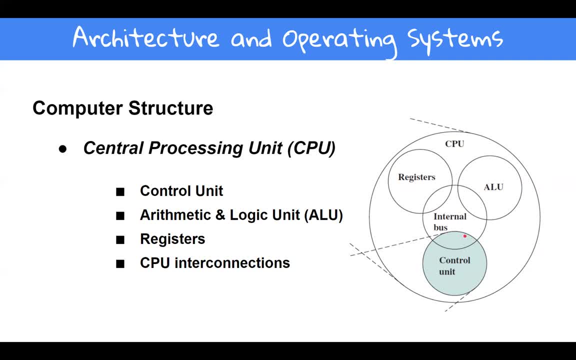 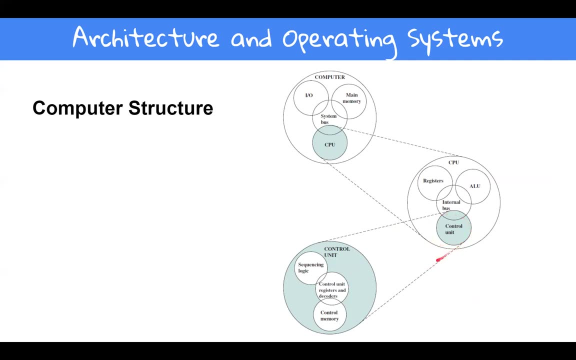 Some mechanism that provides for communication among all, Among the control unit ALU And the register. This is the second level of computer structure. As you see, We can actually study the control unit That we will do, Which is about controlling register. 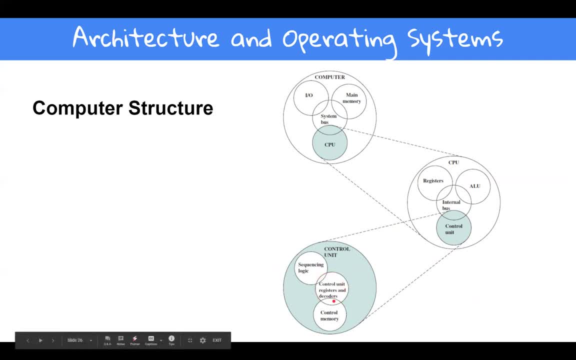 And decoders, Because when we write a code The computer should understand that And then send the signal How computer understand that we are adding numbers Or subtracting. So these signals inside the control unit Will help us to tell the other components. 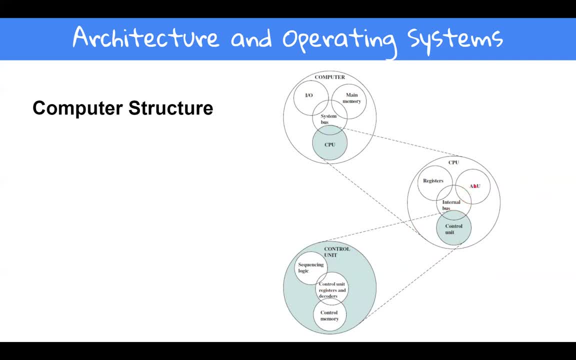 Like ALU That look, This is the adder, This is the subtraction. We need to have a memory And we need to have sequencing logic. We will discuss that later on in more detail As well. So, as you see, 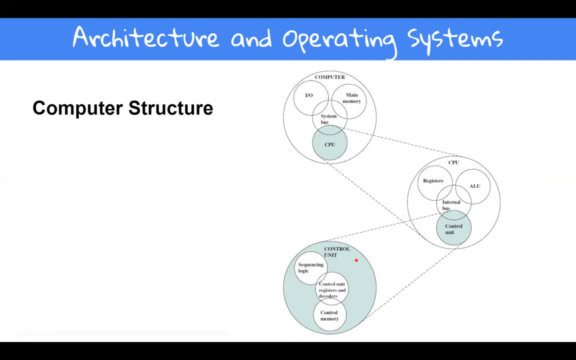 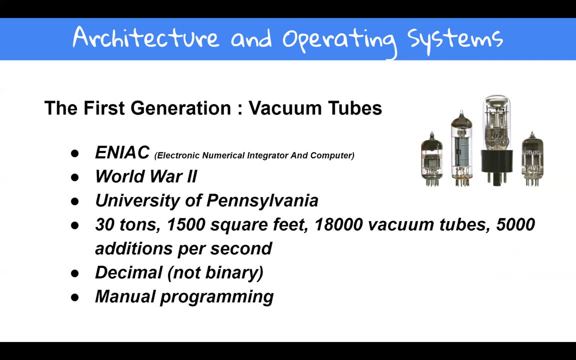 These are the three levels of computer structure That we have Now. You know about the computer structure, Different components. We will discuss the architecture shortly a little bit. But what is important to know what happens. Because, as I said at the beginning, 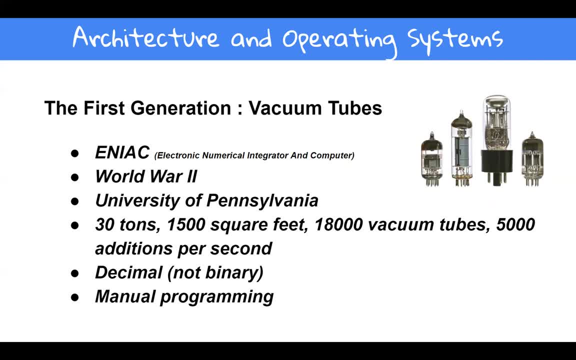 That the computer architecture From a certain time hasn't changed that much The stuff that we need to put together to be able to Run the programs. But let's see how it was. The first generation of the machine Use different organization. 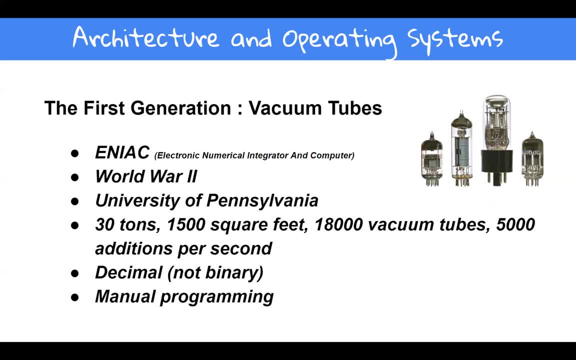 Different components, Called vacuum tube. The machine that Was made Firstly was any Which is stands for what the electronic call electronic numerical Integrator and computer Design and construct, And the university of Pennsylvania Was the very first Computer engineering. 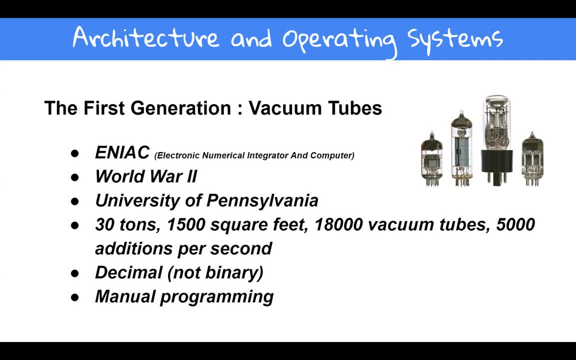 Was the verb, was the words First general purpose: Electronic, digital computer. The pro project was a response to us needs During second world war, The army's ballistic research lab And and and agency Responsible for developing range And trajectory tables for the new weapons. 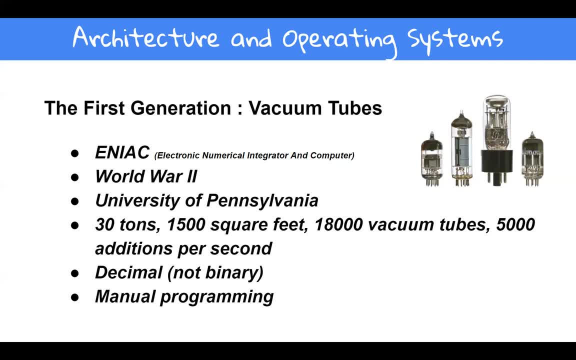 Was having difficulty Supplying these tables accurately And In a reasonable time frame. So they wanted, in the second world war, They wanted to have tables for their weapons To Actually use them. Without these foreign tables, The new weapons and 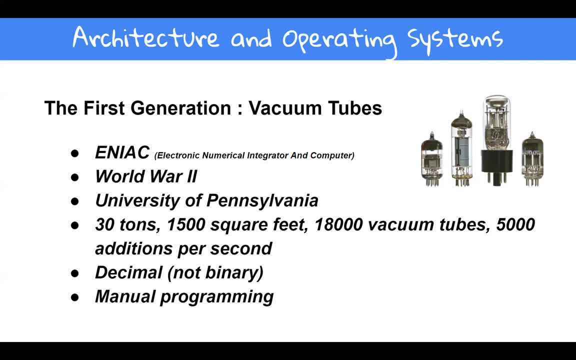 Our theory Very useless to gunners. That's ballistic. research lab Employed more than 200 people Who use desktop calculators. Solved the necessary Ballistic equation To Preparation of the tables For a single weapon Would take one person. 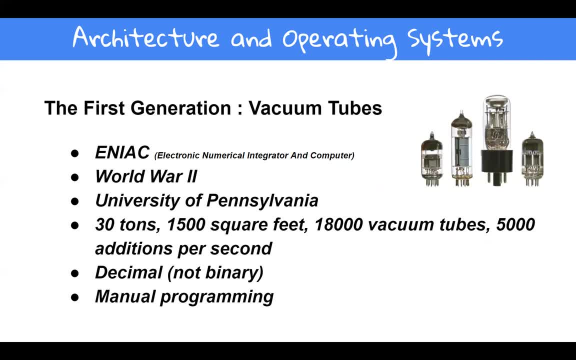 Many hours, Even Days. So The necessity of have a computer Actually was from second world war. In university of Pennsylvania They use This vacuum tube And created the first machine. A professor of electronic engineering at the university of Pennsylvania. 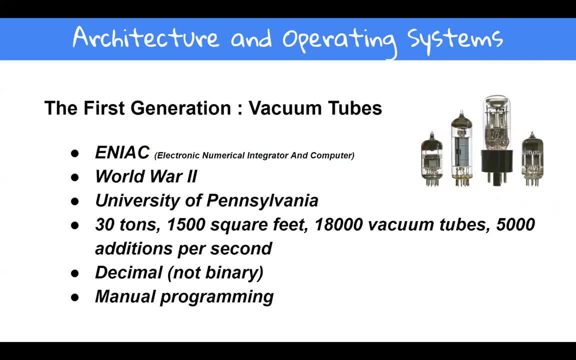 And One of his Students Proposed to build a general purpose computer Using vacuum tubes For That Lab In 1943. The army accepted the proposal And work began On the Machine And resulting The first 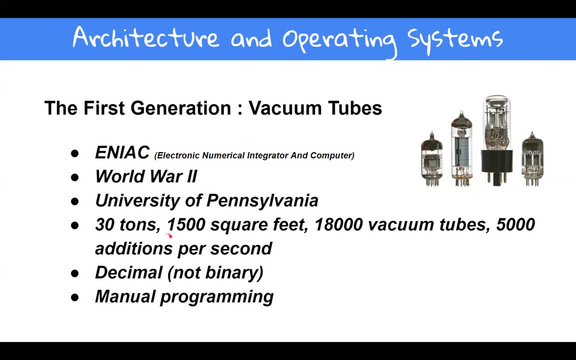 Enormous machine That waited. 30. Tons, Sorry, 1500. Square feet, 18,000. Vacuum tubes And What it does, 5000. Addition Per Second. So that was the first machine. 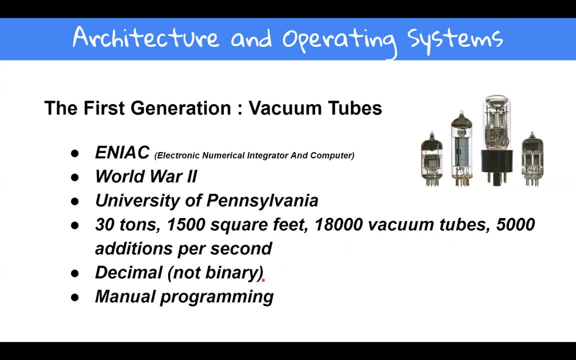 The first machine Wasn't working on the binary system. It falls on decimal. It means that They put tens of these Vacuum tubes Next to each other And when one of them is on, It shows what number that they wanted to use. 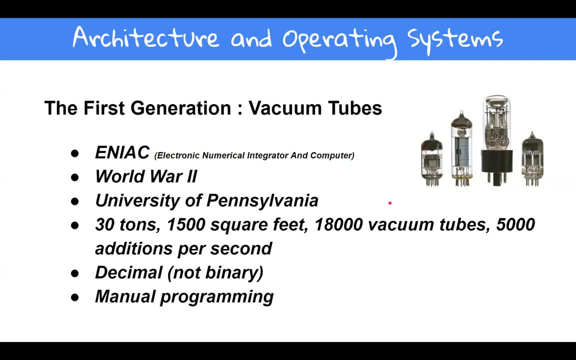 And they've got to put it. I actually put them together, Connect them By the wires Manually, So because of that we call it That machine worked on Manual programming, Because Manually People And Actually 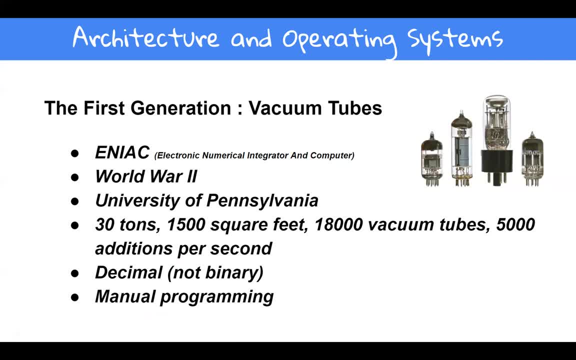 People who work there On that machine Should manually Create The circuit That we use in, For example, And be Actually created In Logically. So they had to put the wire together From one Tube To the other one. 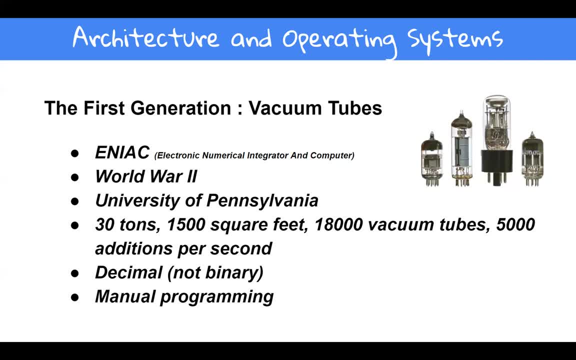 To be able to program. So this is called manual program. But these days We don't do manual programming Because what we do We write A code And the computer Interpret That And create The right Circuit. 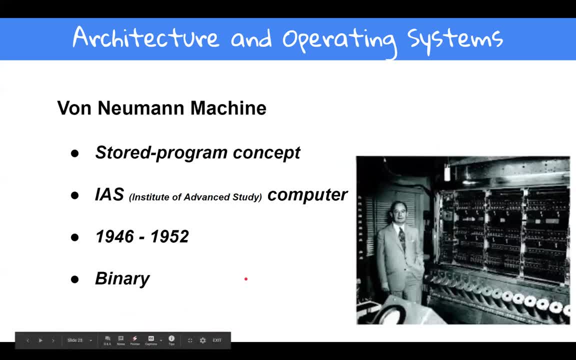 For That operation. So That was the first machine, But There were some problems With that. The main problem Was with Manual programming, And Another problem Was that People Should Actually Write A program. 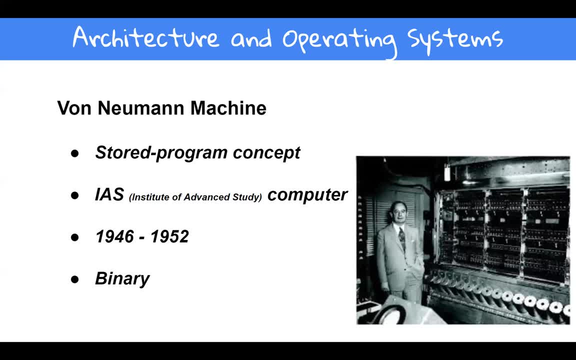 And Then Operate It And Create The Circuit Manually. But Someone Called Van Neumann, As Germans Say. They Thought About A New Machine, Van. 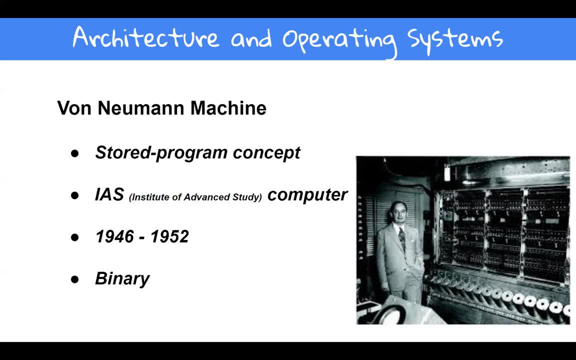 Neumann Machine Or Van Neumann Architecture. The Van Neumann Machine Was Started While Having A New System. That Was The Initial Steps For Developing. 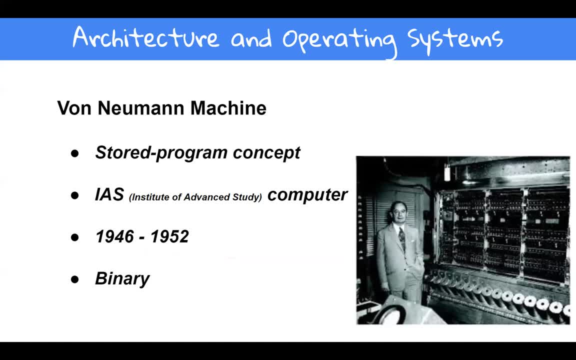 That The Task Of Entering An Alter Altering Programs For The Any One Was Extremely Tedious. The. Not only we should be able to store the data on the machine, but also we should find a way to store the program on the machine as well. 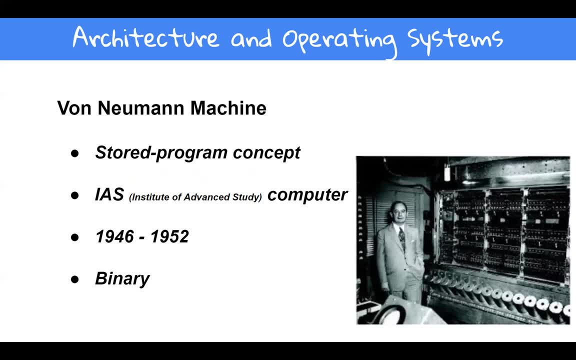 In that case, it's easier for us to do the operation. The idea known as a stored program concept is usually attributed to the ENIAC designer, most notably the mathematician John van Neumann, who was a consultant on the ENIAC project. 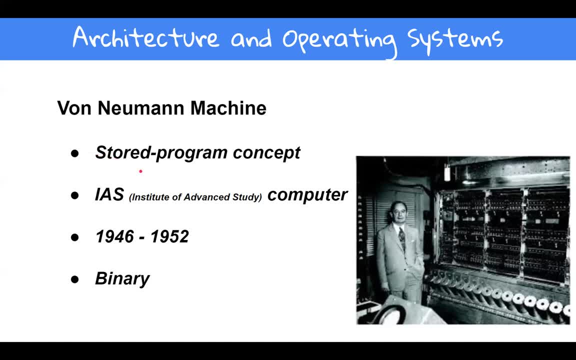 So van Neumann wanted to solve the problem of storing the program and the data both on the memory. So that was the idea of van Neumann architecture. So what he did actually? he created the first program, the first machine called IIS Institute of Advanced Study computer. 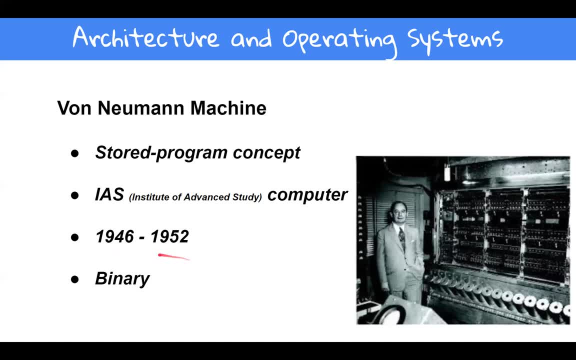 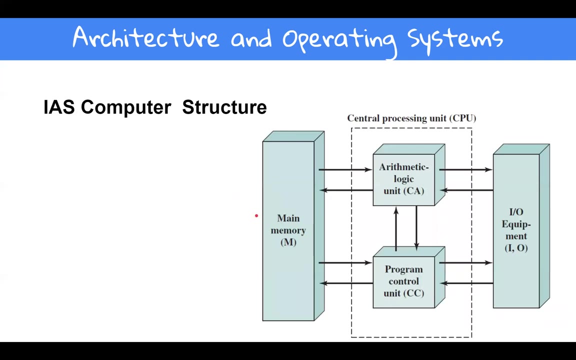 which took a couple of years, six years, to build that machine. This machine works based on binary numbers. The ENIAC was on decimal system but van Neumann was on binary system And he proposed architecture for that. This architecture, or IIS. 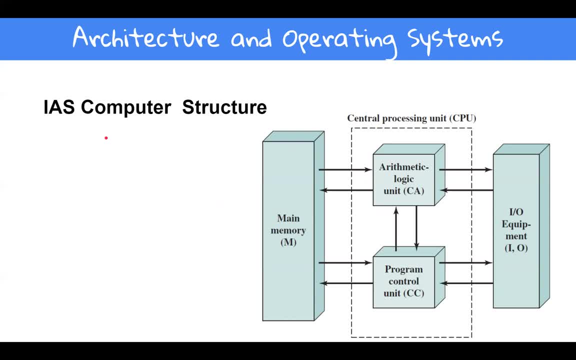 or van Neumann architecture is something that these days, all the machines are work based on that. So this is the structure of this machine: A main memory which stores both program or instructions and the data. We have this main memory to store both data and programs. 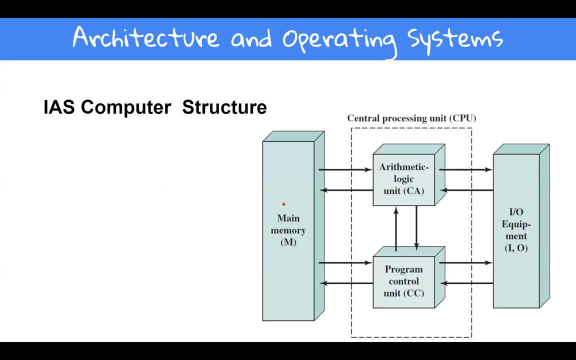 Because of that this is called stored program concept- Stored both of them. It means that when you write a code, for example, X equals Y plus Z, the machine will translate that as an instruction and put it inside the memory. Also, we've got the CPU. 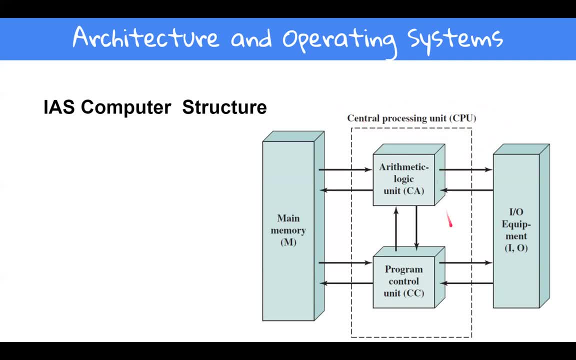 central processing unit In the CPU, we've got the control program unit, CC, and we've got ALU arithmetic logic unit And also we've got input and output devices. So this is the main structure of the van Neumann machine. that we will discuss in more details later. 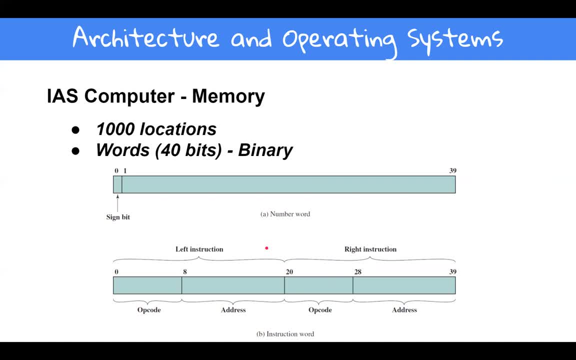 But one thing about van Neumann or IIS computer, about the memory. The memory because I said that it's a stored program concept, So we need to have a memory to be able to store both numbers, data and also the instruction. 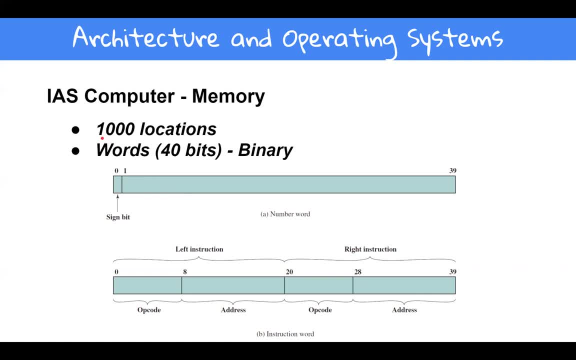 So this memory, this machine memory, has had 1000 locations, from 0 to 999.. We've got two types of words: Word is actually the length of and the length of the memory that we use, that they used actually The number word. 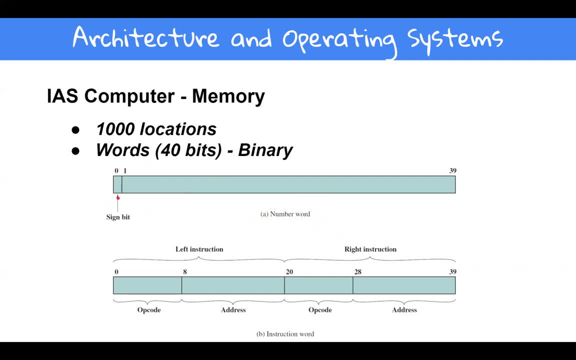 which the first bit shows the sign of the number and the rest for the magnitude. So it uses sign magnitude. This is for storing the number. What about the program or instruction? They use another word called instruction word and they're using two parts. 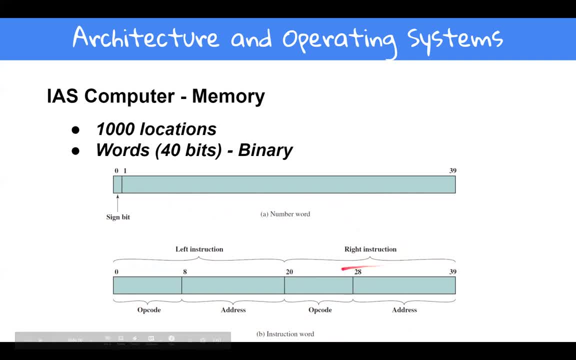 20 bits together. 20 bits together: Right instruction and left instruction. But what it means? they use 8 bits for the opcode and 12 bits for the address, for example, for the left instruction. What it means opcodes? 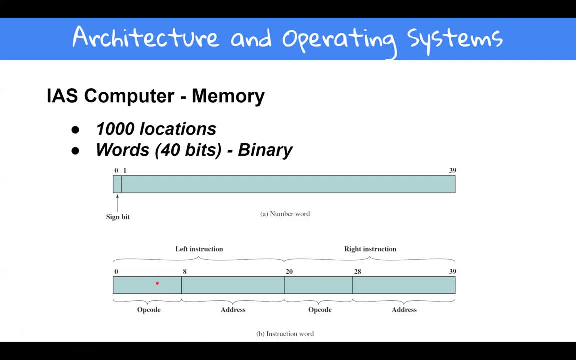 it has some code to. for example, if you want to add two numbers for addition, you store one here. If you want to subtract, you store one zero. It means that the opcodes, or the codes that they use to actually tell computer what to do. 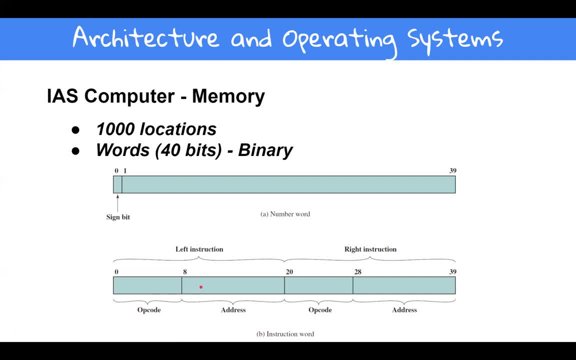 to send a signal based on that And they could save it on the memory. For example, you want to add two numbers. One of them is in the first row and the other one in the second row. first and second row. So first of all, 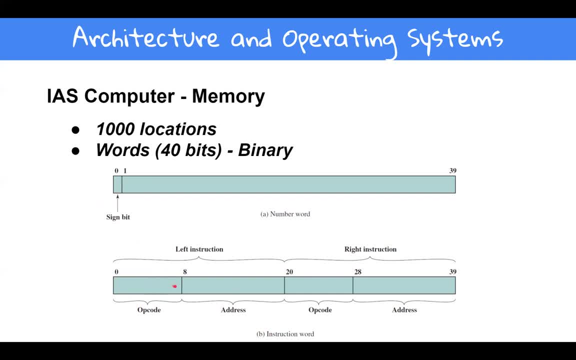 you say that, okay, what do you need to do? Go and read. For example, one is reading a number, Read the first one. The second instruction: read the first row. So you've got to give the address here. Then second instruction is to add: 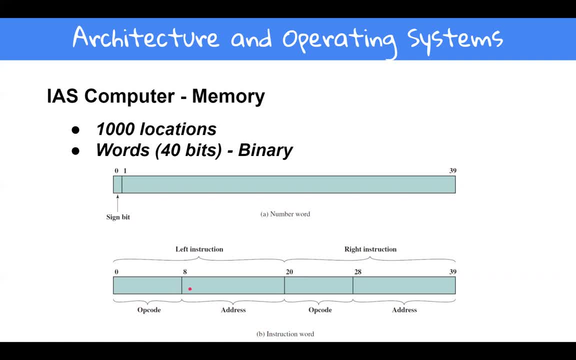 For example, adding the code for adding is two, Adding the second number, So you give the address. So as you see here you could address the memory and tell computer what to do using this opcode. We will discuss that definitely in more details. 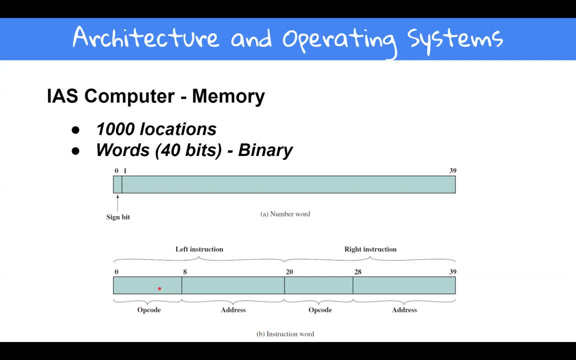 when we discuss fetch execute sign. But what is the most important thing that Van Neumann or in IIS computer they thought about store the data and instruction, both of them on the machine in this way, Storing the data using sign binary.